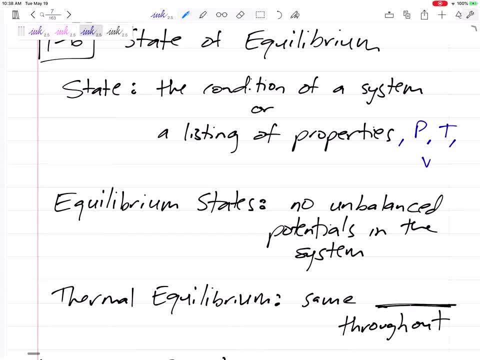 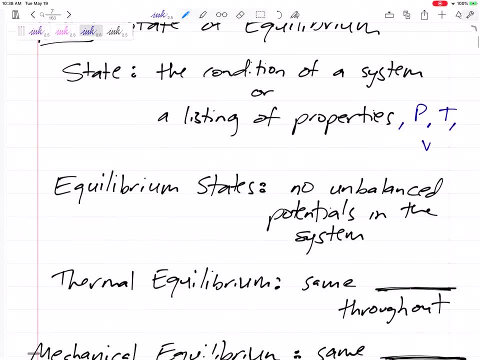 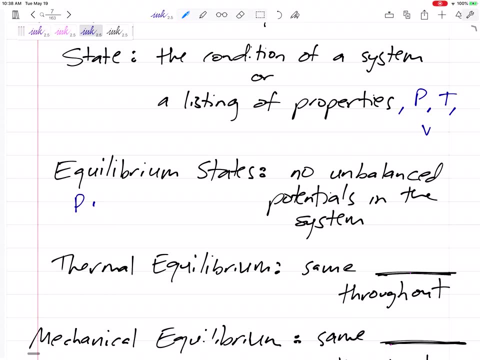 So, if I can list off all the properties, or some of the properties, of my system, that is the state of my system And an equilibrium system. equilibrium states says that there are no unbalanced potentials in the system. That means the pressure is the same. 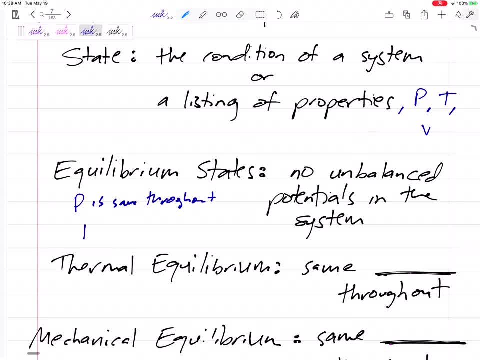 throughout and the temperature is the same throughout, Meaning. okay, the temperature on the left-hand side of my tank is the same as the temperature on the right-hand side of my tank Or, this is more important, the temperature on the bottom is the same as the temperature on the right-hand side of my tank. 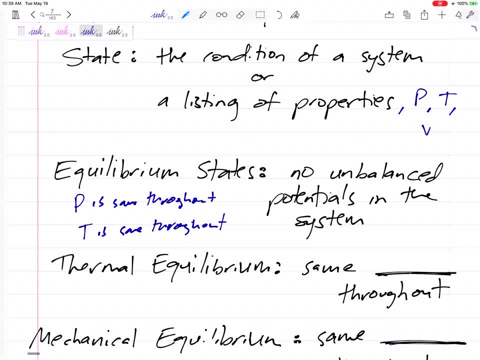 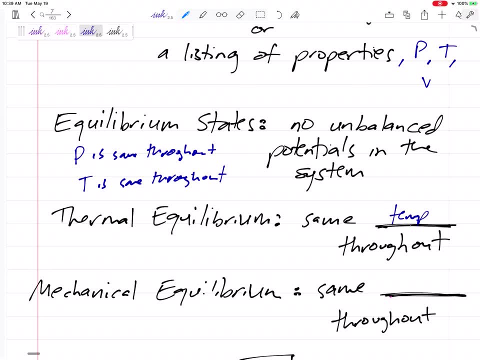 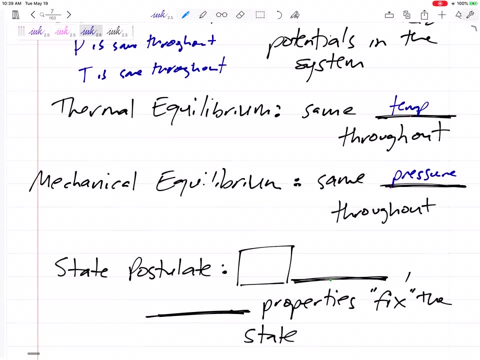 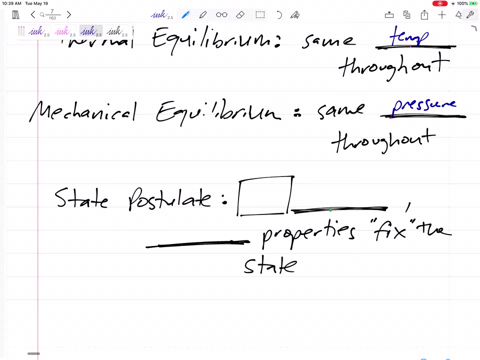 So if it is in equilibrium, we're assuming that the temperature is the same throughout. the pressure is the same throughout. Thermal equilibrium is that the temperature is the same throughout. Mechanical equilibrium is saying that the pressure is the same throughout my system. Okay. And this important state postulate says that we need two independent 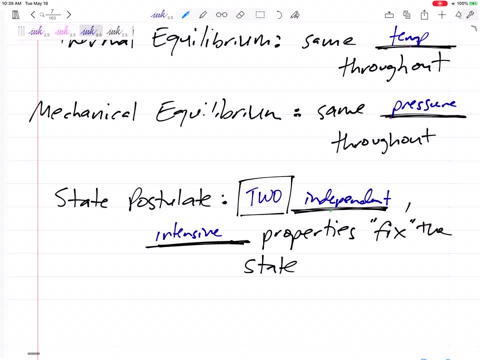 intensive properties to fix the state. All right, Two independent intensive properties to fix the state. For example, if I know the pressure of a system and I know the temperature, then I can find everything else, Then I know the state. We have some equations where we can find everything. 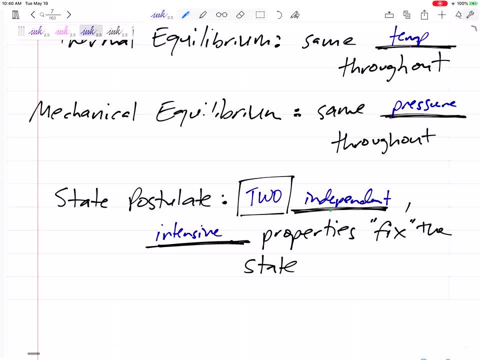 else, As long as we know two things: the pressure and the temperature. If we just know the pressure, then we may not confine the energy, We may not confine all the other properties. But if we know two things, like the pressure and the temperature, or the pressure and the volume or the temperature, 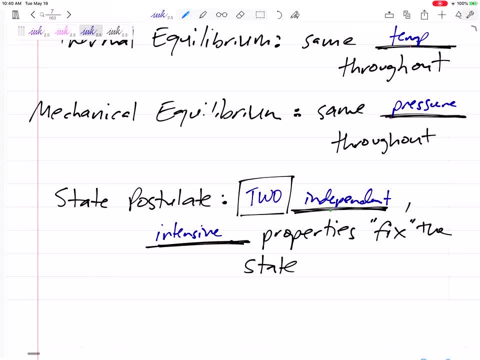 and the volume, things like that, then those fix the state. That's the state postulate. So basically we're kind of looking for two properties to fill in the other properties. As far as properties like entropy, enthalpy, we'll talk a lot Specific volume, temperature, pressure, things like that, If we know two of them. 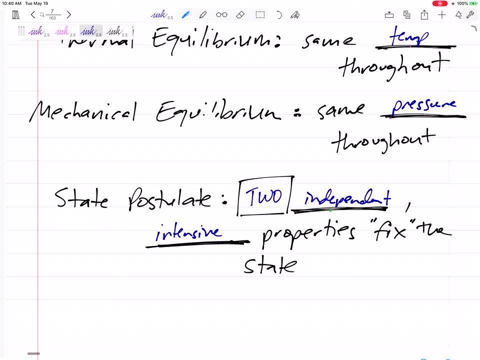 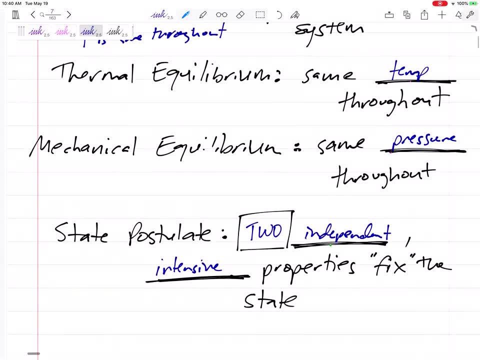 we have some tables in the back of the book. We have some formulas to find the other properties. We're looking for two intensive properties that fix the state, That's the state postulate.